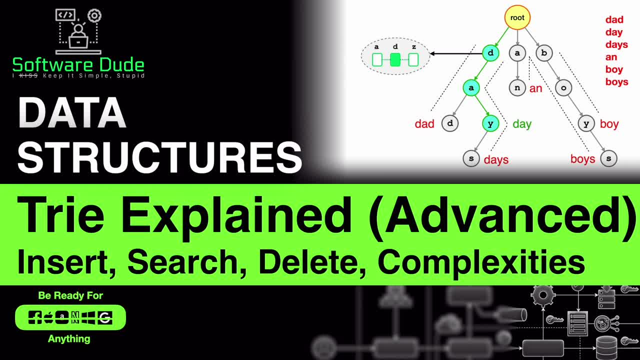 underlying data structures. that is asked in interviews. Most of the problem solvings that you will do based on various types of problems, like based on strings, definitely use TRY data structure. underneath We are going to discuss and explain the entire TRY data structure and also look at all the operations: insert, delete, search and also delete has multiple cases, like 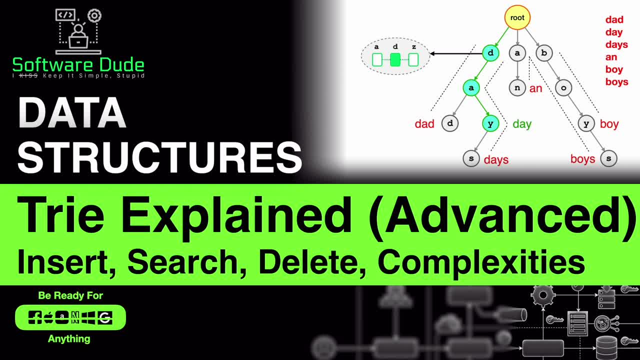 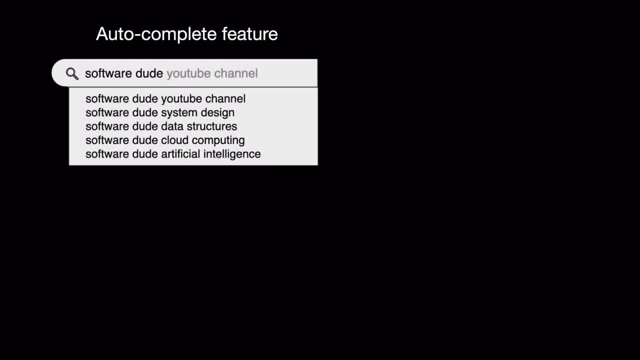 it is a complex data structure, So we are going to walk through all of them at the end of the video also, So let's get started. So now, first let's look at what are the kind of features. So we know autocomplete feature, for example. Whenever we are doing a search, we know how autocomplete works. 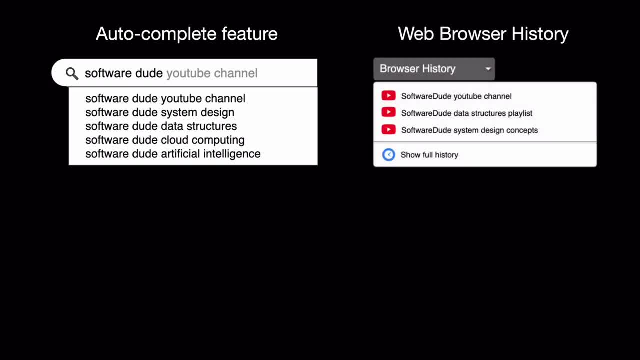 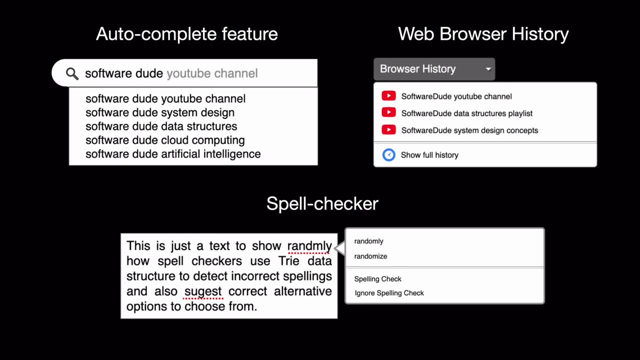 Or let's say there is a search, So let's say there is a search. So let's say there is a search. The web browser history, or we know of spell checker. What do these have in common? They all, underneath, use the TRY data structure And there are multiple other use cases in the real world. 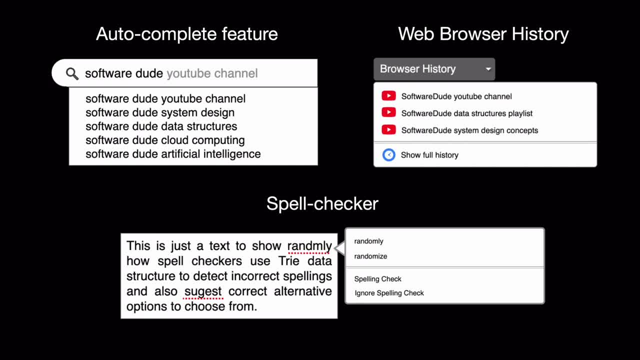 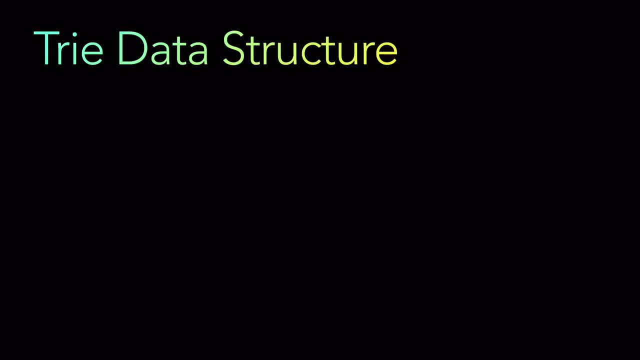 also And, like I mentioned, it's one of the most commonly asked interview questions. So what exactly is TRY data structure? TRY data structure is a tree based data structure which is basically to store and efficiently search and retrieve strings Right. Primarily, it is based on strings. If you look at a TRY data structure something like this: 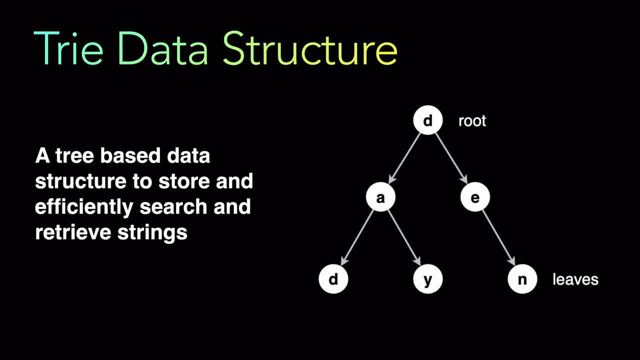 Right, Which is a tree? It has a root, It has leaves, It has children, It has everything that a tree data structure has. But what it stores are characters within each node. But it is not exactly one character at a node And we are going to look at how the node is next. A TRY node. 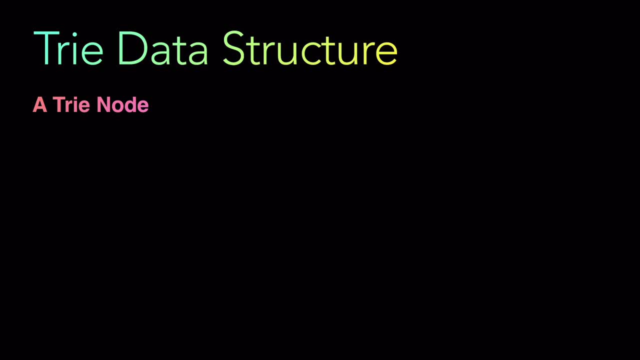 Let's say so when we are talking about strings, Right At that point of time. strings can like characters can be of anything. It can be case sensitive, It can be A to Z. 0 to 9 can also be considered as characters within a string. 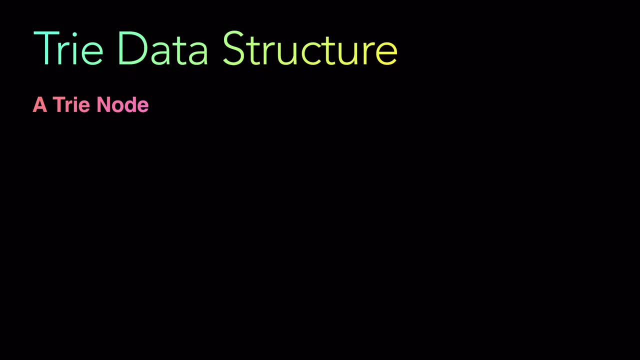 Then there are alphanumeric characters, Then there are symbols, Right. So, for the sake of simplicity, let's say that our TRY data structure will only contain small alphabets, Right- A to Z, small alphabets. So let's say it only: our data structure only contains A to Z in small A node in a TRY data. 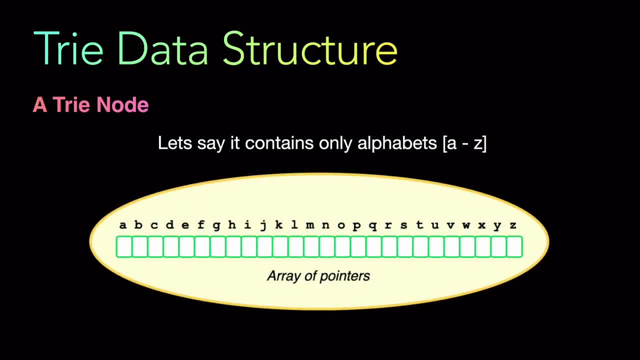 structure is something like this: Right, Which is basically every node has an array of pointers for each of the characters that you are going to store, Right, So at any node it has so say, let's say, we are storing small alphabets, A to Z, Right, So we? 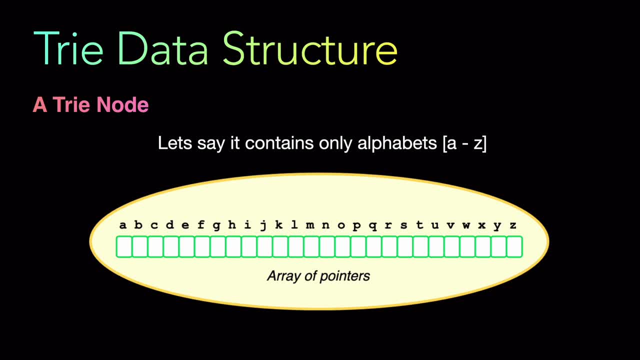 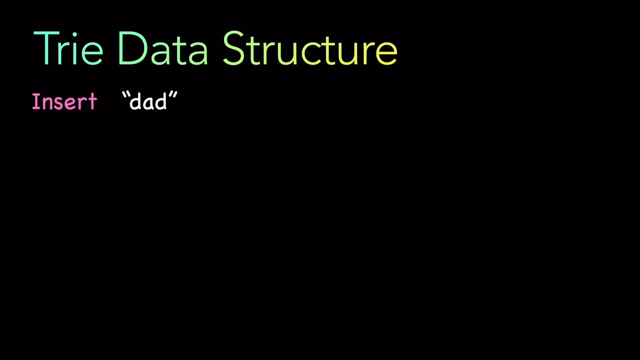 are going to have 26 array pointers each of the positions filling A, B, C up till Z. Right, Let's look at if we have to apply this and let's look at all the operations. First, let's say that we are going to insert a word called DAD. Right, Now we already- it's a TRY- data structures. We. 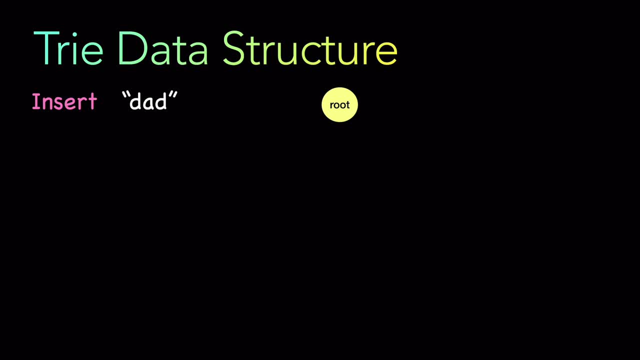 already have a route from the route. We are first going to insert the letter D Right. So how will that get inserted? A node that has all the character array pointers A to z, But D is the that is filled right. that indicates that that node only contains d character right. and but is d a. 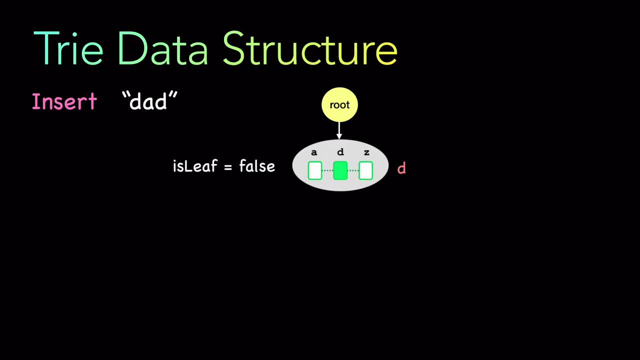 leaf in the tree. no, so we mark it as false. and is only d a word right? we are not considering that as a word, so we are going to mark it as our word count is zero. the next character is a right. so now, from d we are going to move to the next node. insert another node and that node itself. 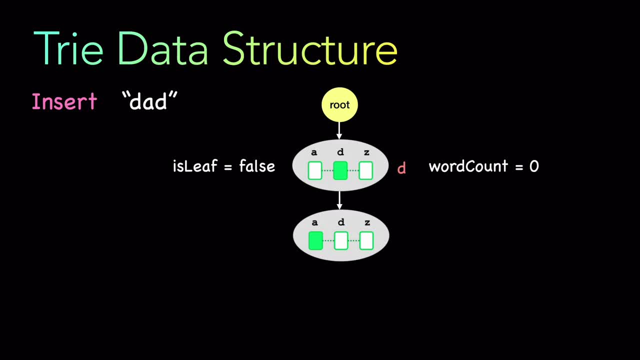 also is going to contain 26 characters, 26 array pointers from a to z, but only a is going to be filled, right. but is this a leaf node? no right, so it is left is false. and are we considered considering d, a, like da, as a word? no right, so word count is also zero here. now the third character is: 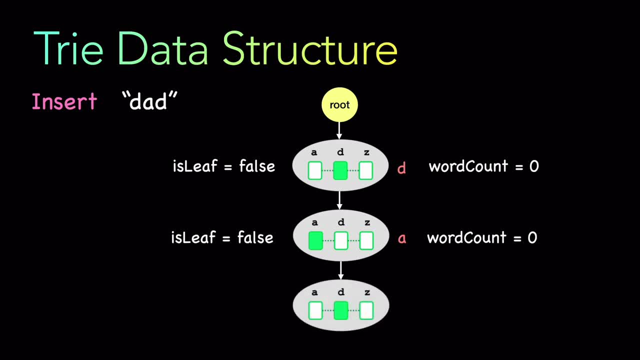 again d. we are going to insert another node and again fill the position of d in that array of 26 pointers. now we have inserted dad, right, and is this a leaf? yes, it is a leaf, right. and are we considered dad as a word in our tree? yes, we are considering that as a word in our tree, so we are going to mark this. 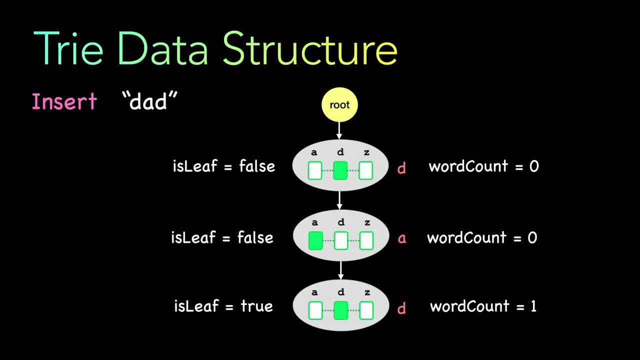 as one, right. so at the like, d, a, d, the third character, which is d. at that point of time, we are marking that we have a word there starting from root. so if it, if anyone travels from root, uh, the third node, d. we know that there is a word starting from there, right, so that word is that: 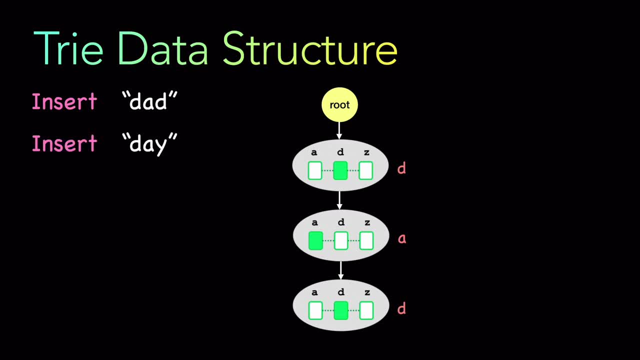 now let us take another example on top of this itself. let's say we are inserting d, we already have dad in our tree right now. let's say we want to insert d and notice d a is already there right in the, in the, in our existing tree. so dad and d a y. so the only difference is the last character. 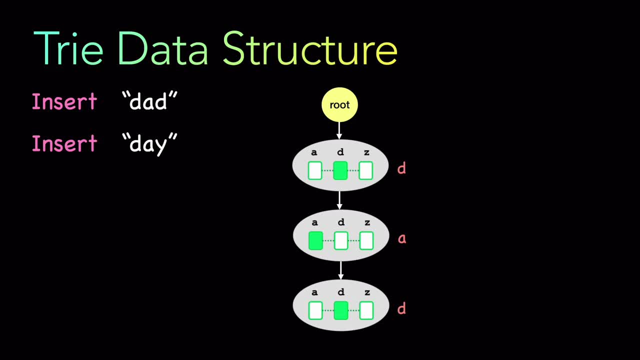 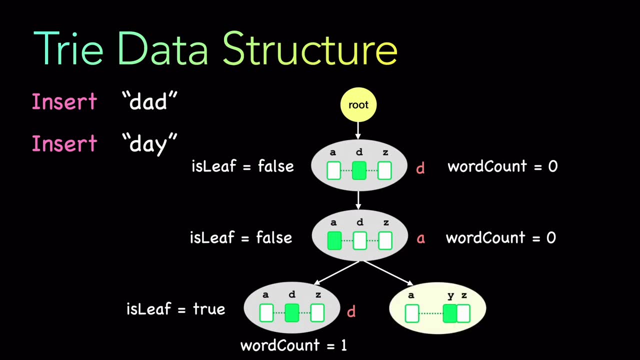 which is y in the existing tree right. the only difference is the last character, and we are going. we already have D, we already have A, so that means we only need to insert Y. How are we going to insert Y? Yes, it is after A. we are going to insert another node and fill the position of Y as. 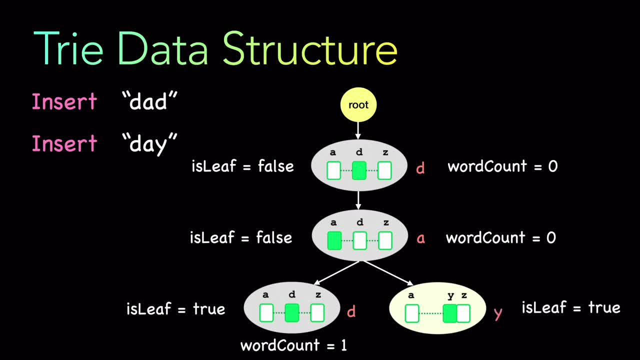 2. And is this a leaf? Yes, it is a leaf, and we are going to mark the word count there as also 1.. So whoever is traversing the tree, if they are looking at only the first node, D, they are going to say that it is not a word, it is not a leaf. If they are looking at D A, 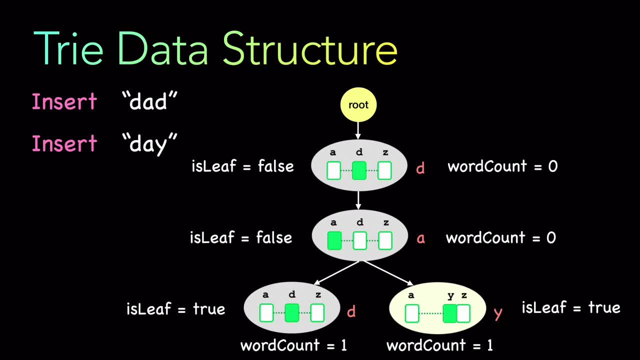 DA, it is not a word, not a leaf. But if they are looking at DAD, yes, it is a leaf, and at that D also we have a word. If they are looking at DAY, Y, Y is a leaf, and at Y also from root. 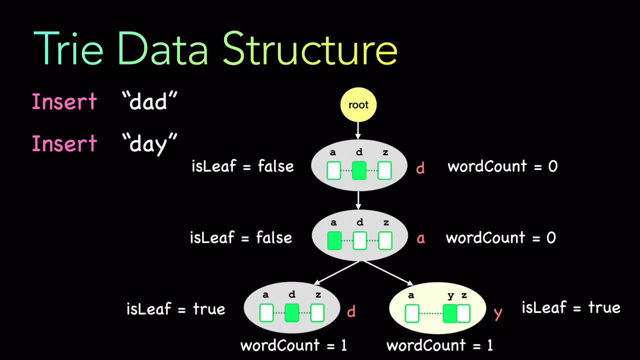 there is a word day, So that is how the tree is getting constructed. Now let us look at a search operation. Interesting because search is one of the most important operations That you are going to do, because the entire game is around searching. 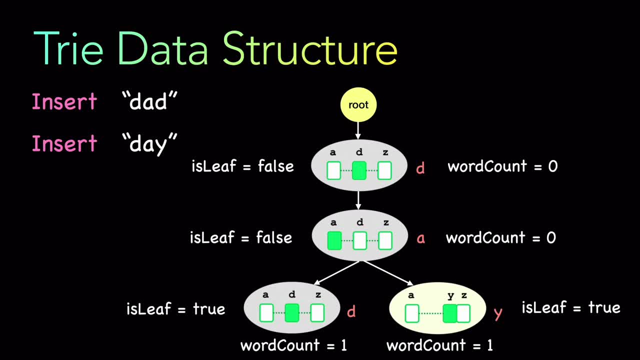 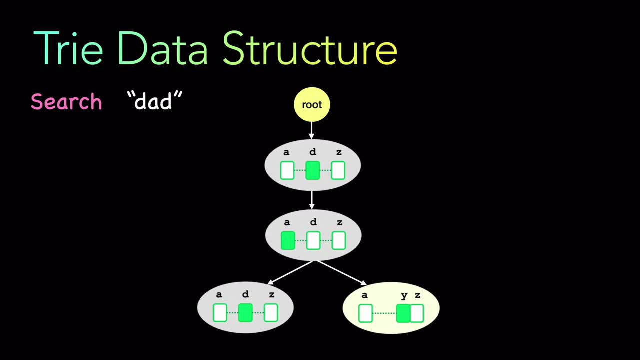 for various kind of applications Search. it is an efficient search algorithm and data searcher. So let us look at searching DAD. Now, if we have to search DAD and look carefully, we are going to search by character, by character. So our first character that we are searching for: 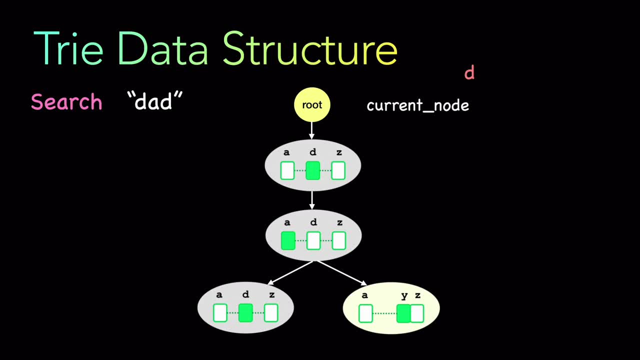 is D and our current node is starting at root node. What we are trying to do here We are trying to figure out from root: is there a child node that has D pointer filled, Which means current node dot. child node of D is null or not null. 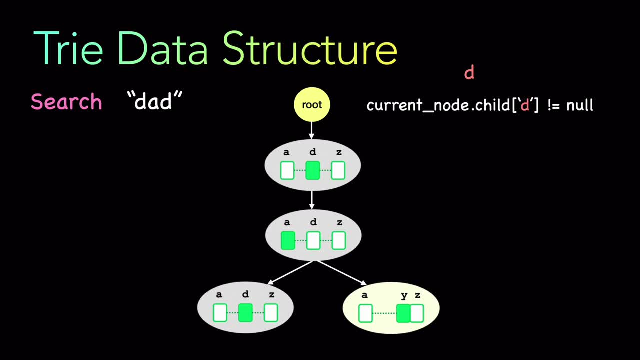 We are looking for something which is not null. Is there one? It is, There is, So we get the D and our current node moves to that child. What is the next character that we are looking for? We are looking for A Same process continues. Is? 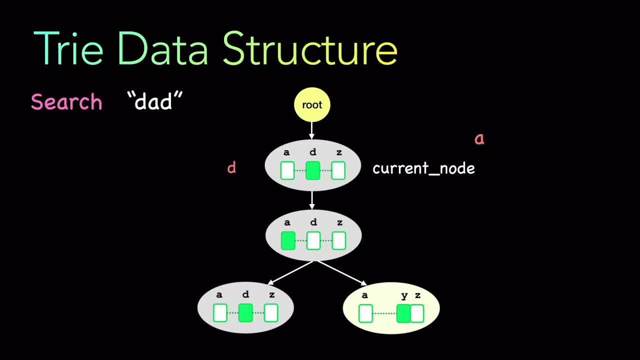 this node? does this node have a child node with a A character pointer as not null Right? Is there? Yeah, there is. So we move our current node to that node and we already got DA Right D, Now we are looking for again D. does this node have a child node where the 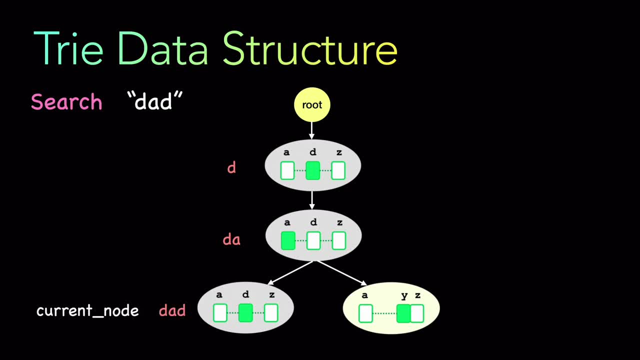 D character array pointer is not null, It is there and we are getting the entire word as a child. So again, complex Ref word as dad and the current moves node moves to, uh, the last d right, i remember at this point of time this node we have marked as a leaf node and we have also marked that this node at this point. 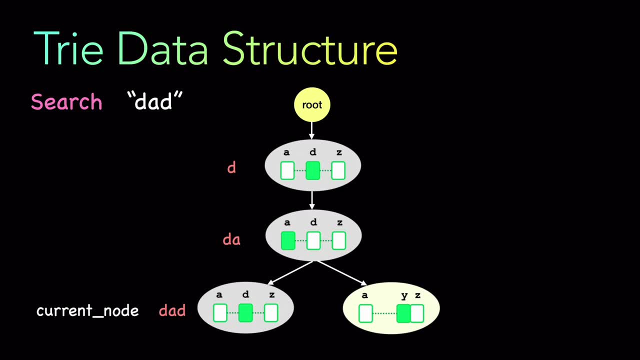 we are going to count word count as one right, so when we reach this point we can figure out that, yeah, we have already got that and yes, there is a word that is ending from root to dad. we the third d, so we already found and searched dad right. also, notice another thing: what are the prefix based? 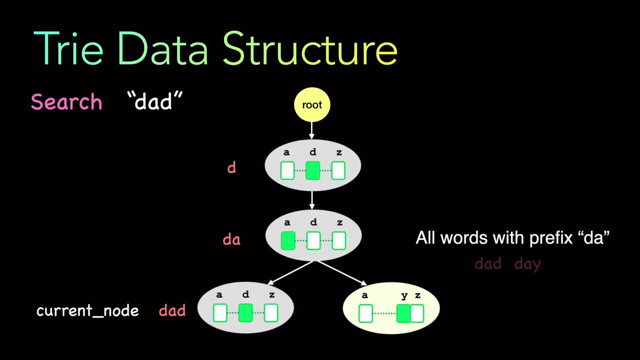 searches right. so all words with prefix d- a right, like dad, and d right, are present. so you can, if given a problem like, uh there are multiple bunch of strings, uh, figure out all the strings which have a common prefix, say whatever, right. and that is so easy here because you already know the 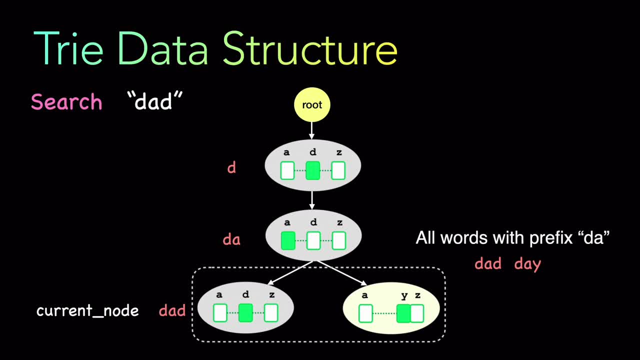 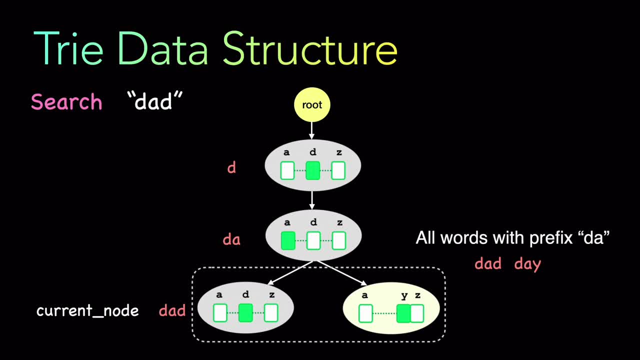 whatever you are searching for, the prefix at that point of time, all the prefix at that point of time, all the prefix at that point of time, all the children that are children, that are children, that are uh uh uh. at this point, with the prefix after the. at this point, with the prefix after the. 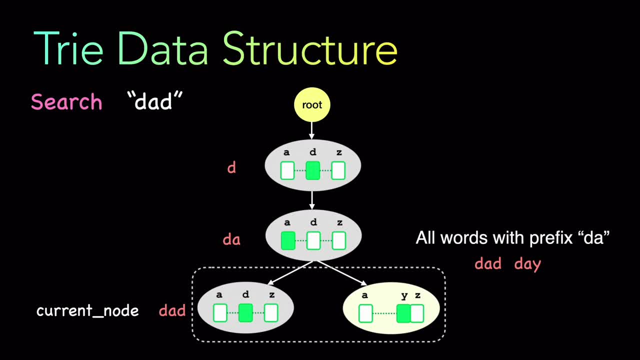 at this point with the prefix. after the prefix are all the words that are there. prefix are all the words that are there. prefix are all the words that are there. right, so it's very easy. so, if the question right, so it's very easy. so if the question 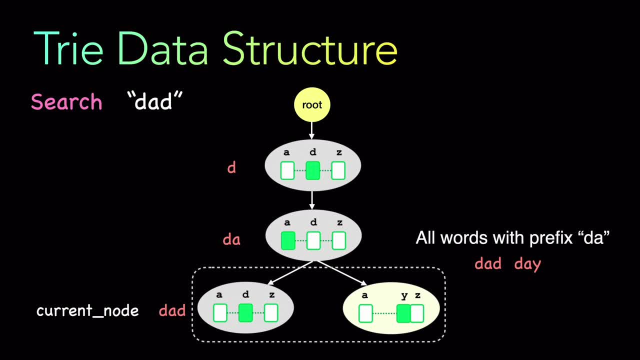 right, so it's very easy. so, if the question is how many the number is the number of, is how many the number is the number of, is how many the number is the number of children, what are the words you can? children: what are the words you can? 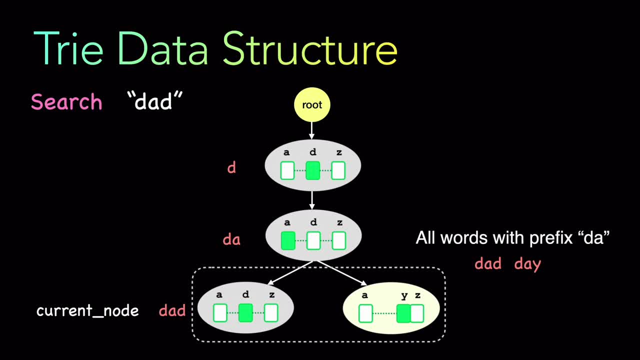 children. what are the words you can traverse one? get the words right. traverse one, get the words right. traverse one, get the words right. so that search now let's look at delete. so that search now let's look at delete. so that search now let's look at delete right. so for delete we are going to take. 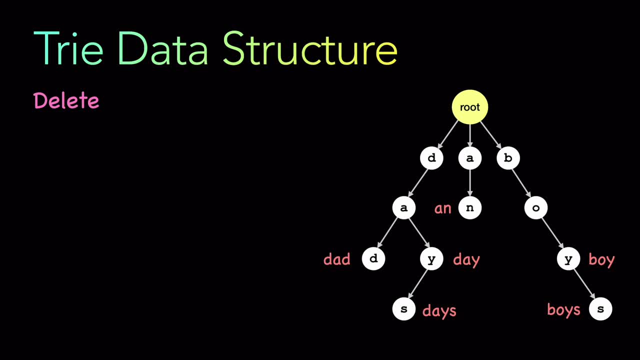 right, so for delete. we are going to take right, so for delete. we are going to take a complex tree and we are going to a complex tree and we are going to a complex tree and we are going to consider that this tree has uh, consider that this tree has uh. 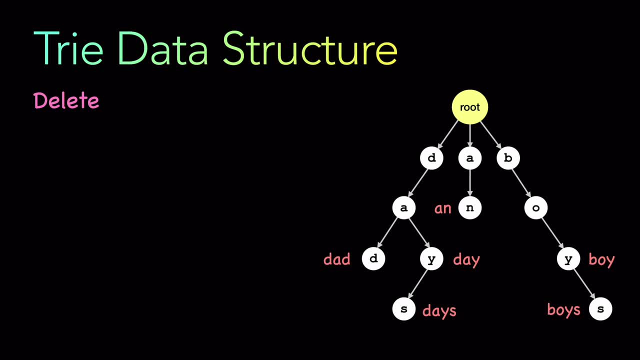 consider that this tree has, uh, six words, right. so our try data structure: six words, right. so our try data structure: six words, right. so our try data structure: currently has six words. currently has six words. currently has six words. now delete, like i mentioned. has very. now delete, like i mentioned, has very. 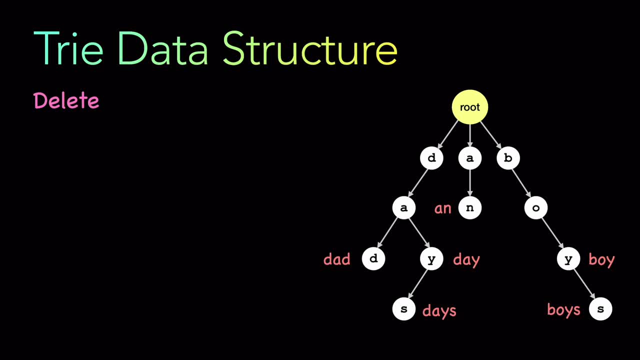 now. delete, like i mentioned, has very complex operations, which is where some of the senior engineer or SD2 level questions are around. delete, where, basically, you have to reconstruct the tree. That is because of the complexity that is there. So we need to understand what are the four cases? There are multiple cases. The first case is the word that 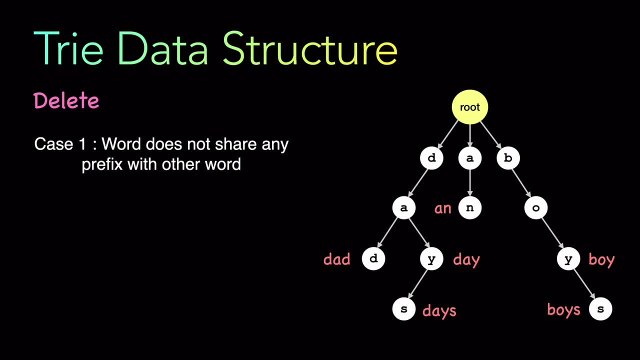 you are going to delete does not share any prefix with any other word. So basically, for example, say: and in the tree that we have and is not shared with any other because we are not considering a as a word. The only word is and From root to n. that entire thing, That and word is not sharing. 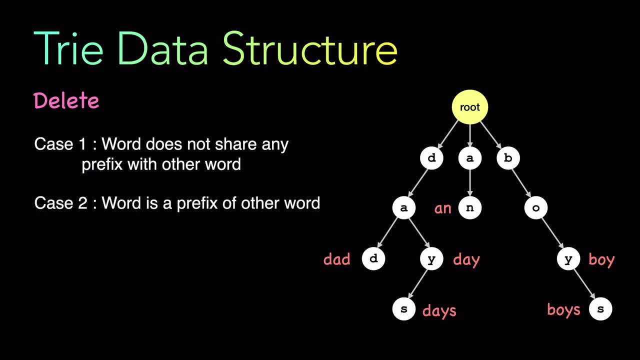 prefix with any other word. Case 2 is the word is a prefix of another word, For example boy. on the right hand side, the entire word is a prefix of another word, which is boys. So that is another case. If you have to delete boy, how will you do that? 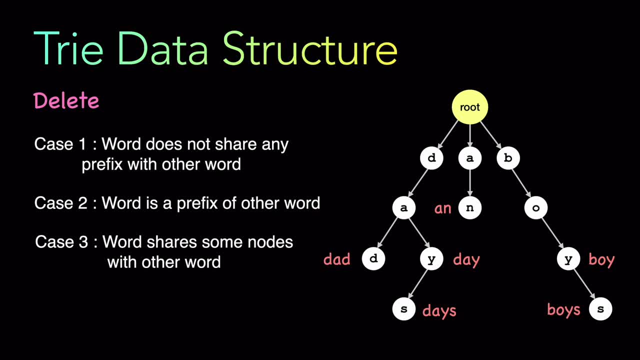 Third case is a word shares some of the nodes with other nodes. right for a other word, like, for example, if you want to delete dad, right, so in dad, d, a, da is the common part. it is sharing the d and a, the first d and a nodes with other words like day and days- right. so if you have to delete dad, how will we delete that? 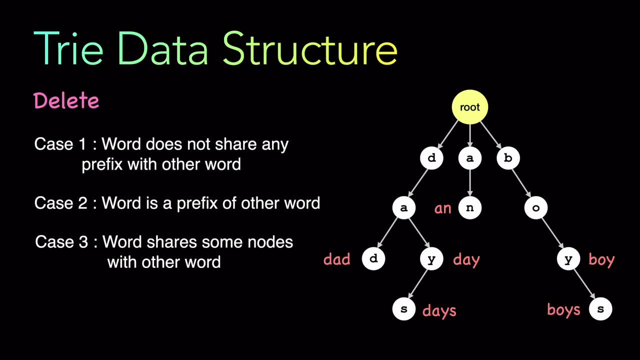 without disrupting day and days right. and the fourth case is the other word is a prefix of this word right. for example say we want to delete days, right, but day is a prefix inside that right. so if you have to delete days, how will we delete days without disrupting day? right, there are four. 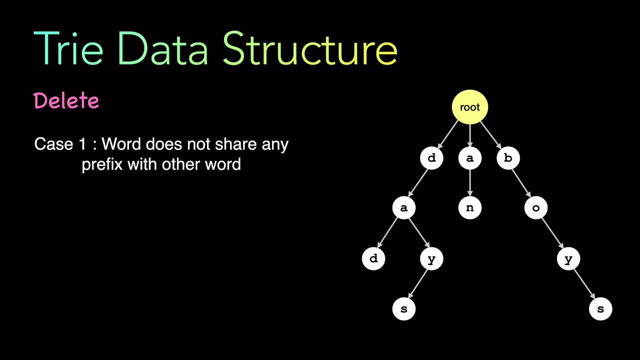 cases. so let's take case by case. in the first case, what does not share any prefix with the other word, right so? which means, like we mentioned, we have an here. since it doesn't have any prefix, our straightforward solution here is: we'll delete all the nodes, right, so it doesn't impact. that's. 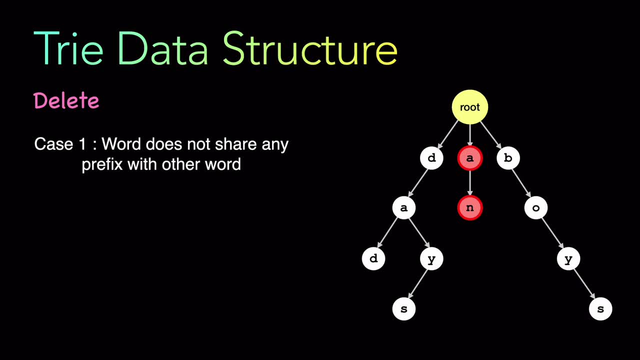 the only word and we can delete the nodes to remove the word from our try data structure. the second case is word is a prefix of other word, right. for example, if we are considering boy, right, boy is a prefix of another word- boys, right. but we know that. to add this, 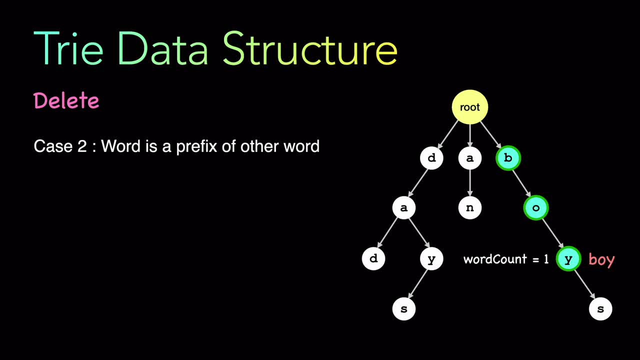 node. we are going to have a prefix of other word, right, so we are going to have a prefix of node. our word count is one. so what is the solution? how we can delete the word boy from our tree without disrupting boys? right, that's the way to do. that is, we don't delete any node, we just 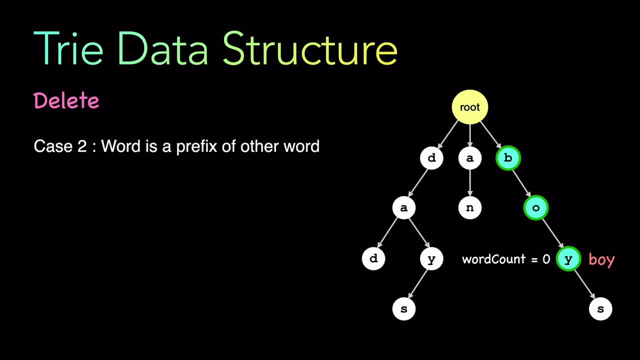 mark the word count as zero. that word count is the variable that is pointing whether we have a word ending at y, starting from root. right, if we are saying that there is a prefix of another word, right, so we are going to have a prefix of another word, right? 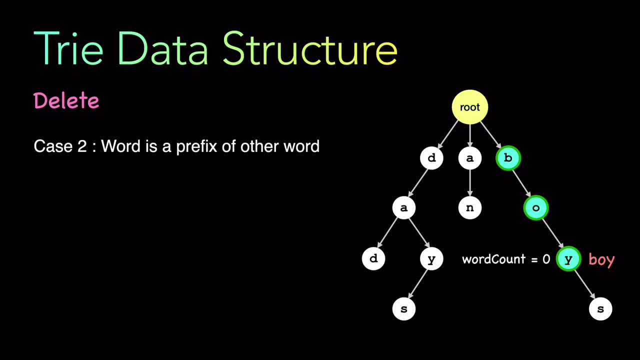 there is no word. so that basically means that we are not considering boy as a word in our try data structure. the letters can be there, but it's not exactly a word, right? so that is case two. now let's look at and word shares some nodes with other node right, like for example: 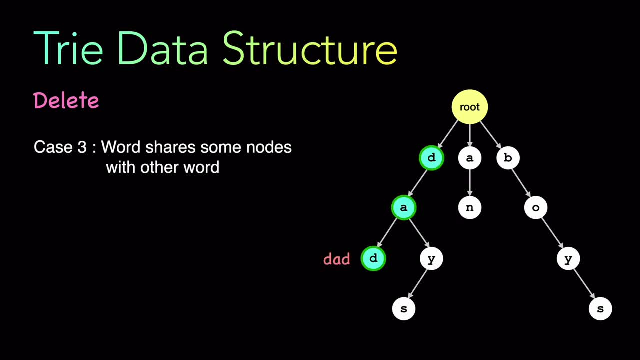 dad. like we discussed in dad, the d and a, the first d and a is shared with other words like day and days, right, so how will we delete dad without disrupting day and days? so the only thing that is not common with other words is the third character, which is d, right, so if we just delete